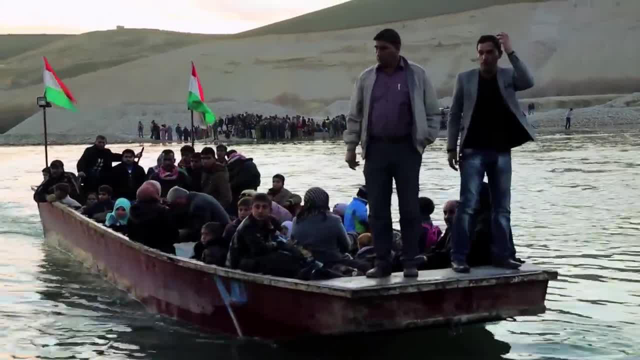 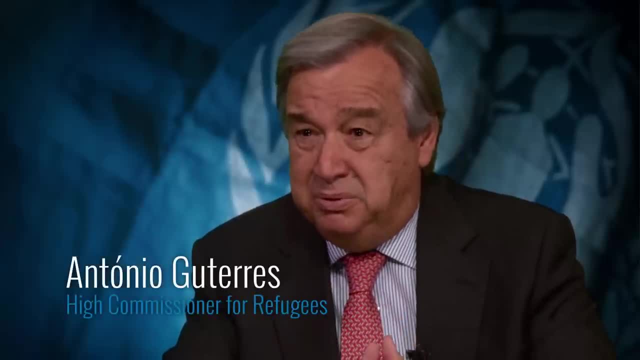 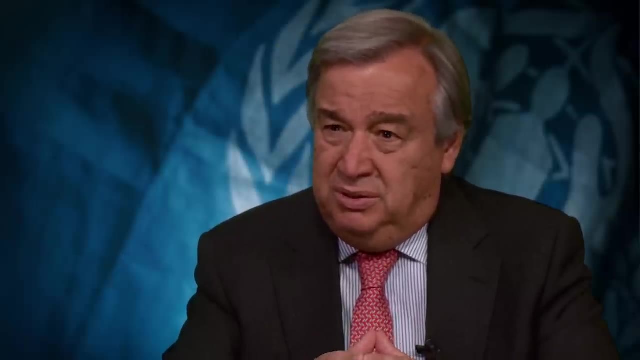 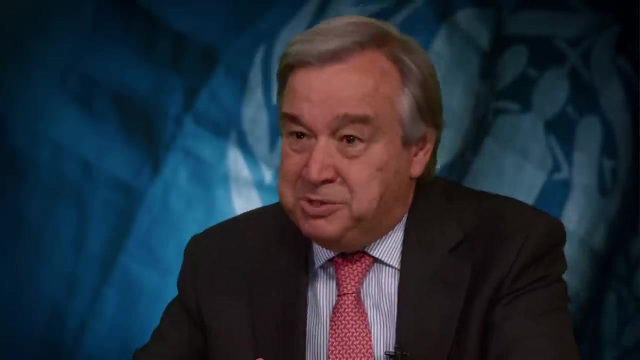 more than in 2011.. If we have, for the first time since the Second World War, more than 50 million people displaced by war or by persecution, it's because we are witnessing a multiplication of new conflicts in the world, And the global conflict generates global displacement And, at the same time, 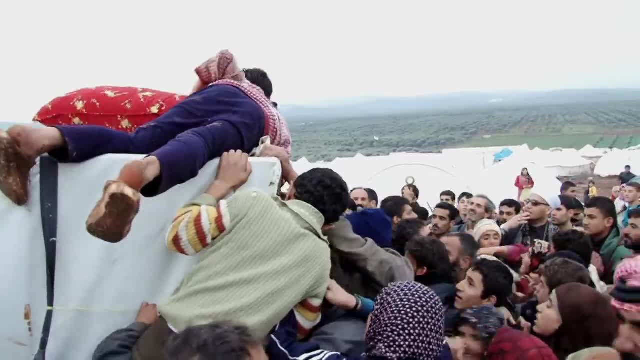 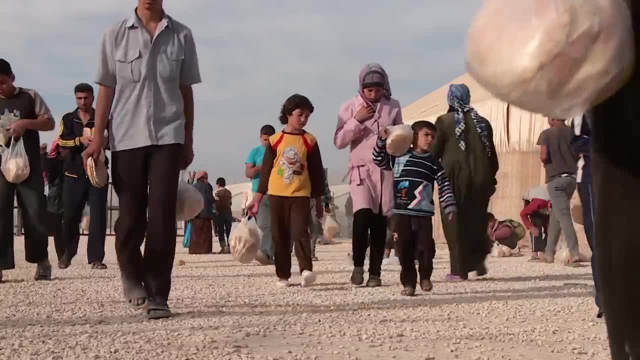 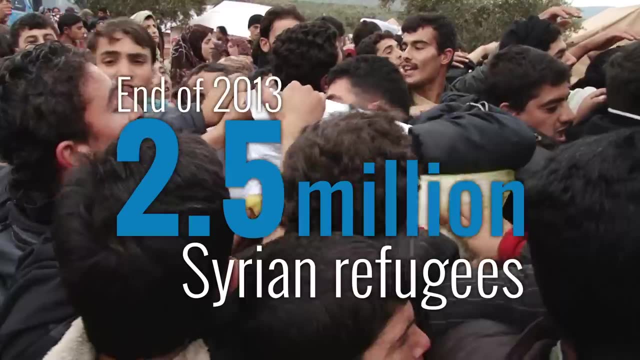 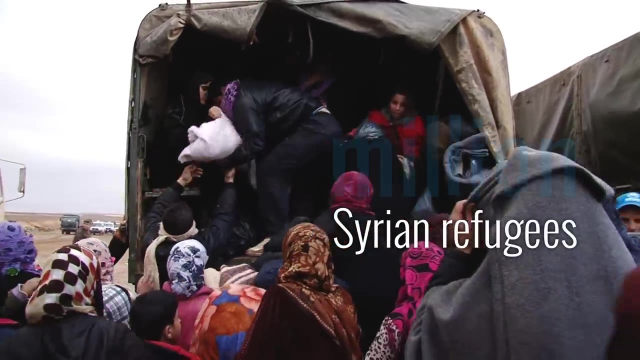 We made a one-year refugee exodus from any country since the Rwanda genocide 20 years ago. By the end of 2013,, refugees from the Syrian conflict totaled 2.5 million. Now they number nearly 3 million. There were also searing conflicts in Central African republic. 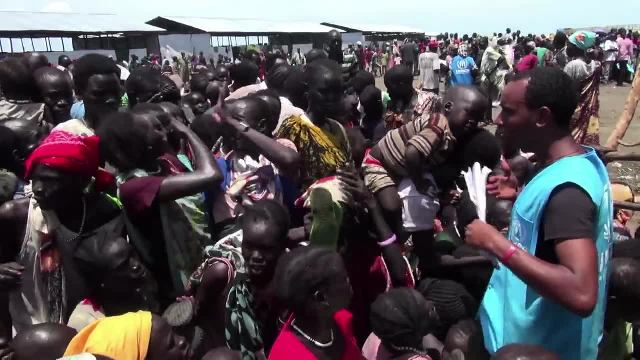 South Sudan, sending rivers of refugees into neighboring countries. Totally durumated, Floating arrivedionen: Jezkel Lossert in Zimbabwe. in Belgium, 9,500 impact in einem pro-Syrian beginning in 2014.. There was new cases in those. 1,500 were residing rubies in the through the abroad borders. 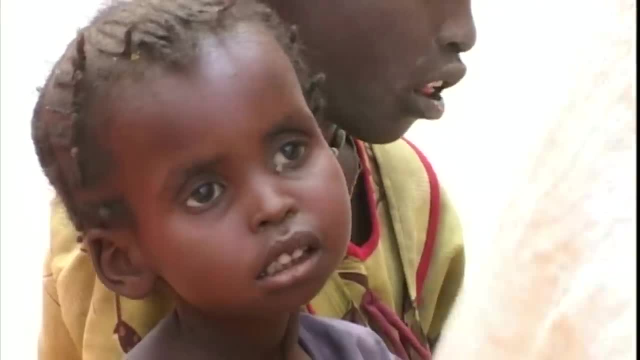 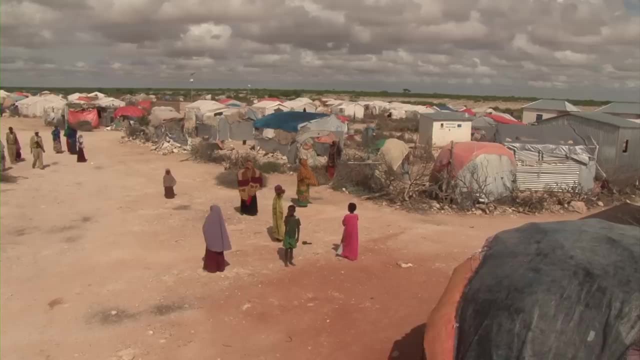 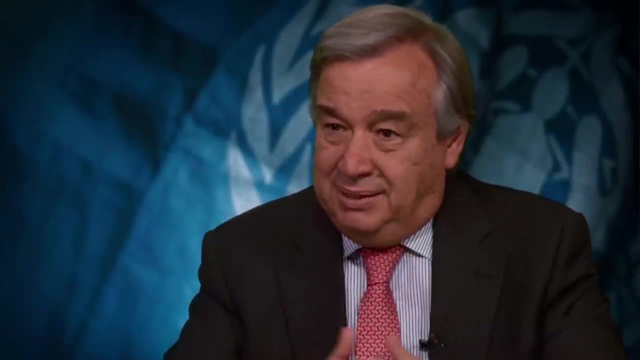 The first Dowry Blockchain, including arms in the不会 I understand, rights would leave that. Cameroon, Chad, Ethiopia And across continents, old, unending conflicts go on. Last year we had a mega-crisis- Syria- with the dramatic humanitarian impact millions. 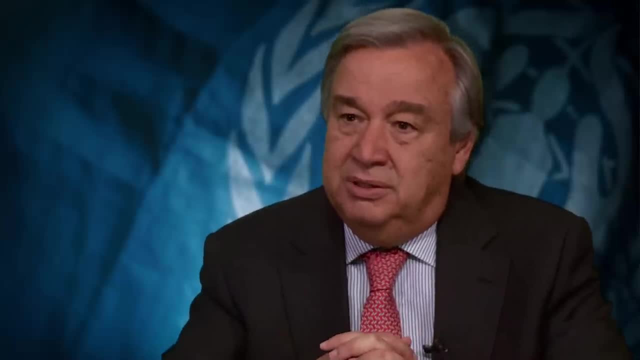 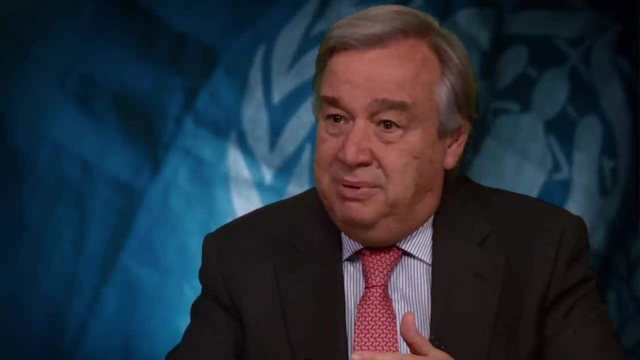 of people displaced inside the country or fleeing the country to the neighboring countries, the physical destruction of Syria. But at the same time we had Mali, Central African Republic, South Sudan, FRED DE SAM LAZARO: 50 percent of refugees are children, the highest percentage. 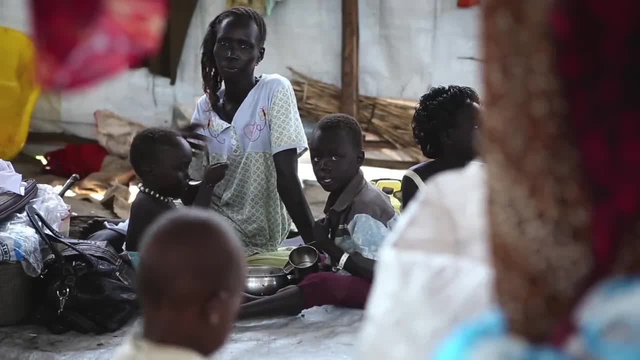 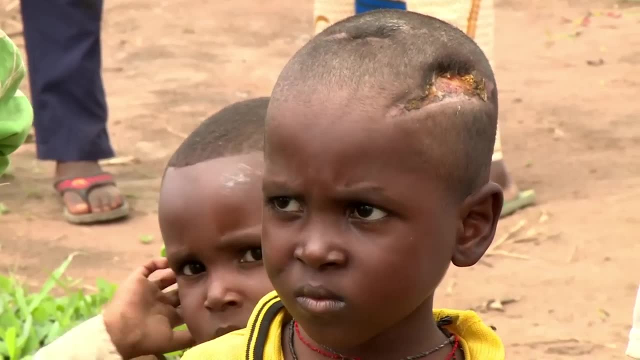 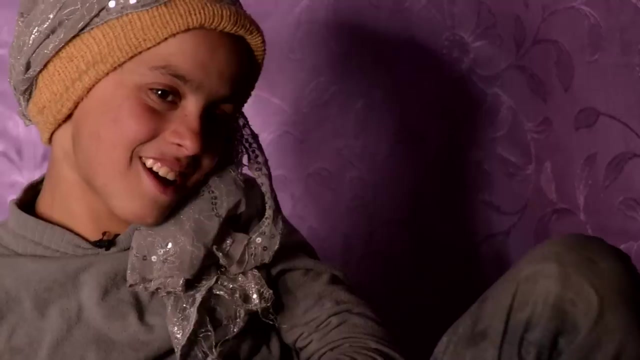 in a decade. Displacement is brutal. Many children stumble into exile barely alive after weeks in the bush. Some, like Ibrahim Moussa, slashed by machete-wielding rebels in Central African Republic, have dreadful injuries. Others, like 12-year-old Hala, must take care of their siblings.